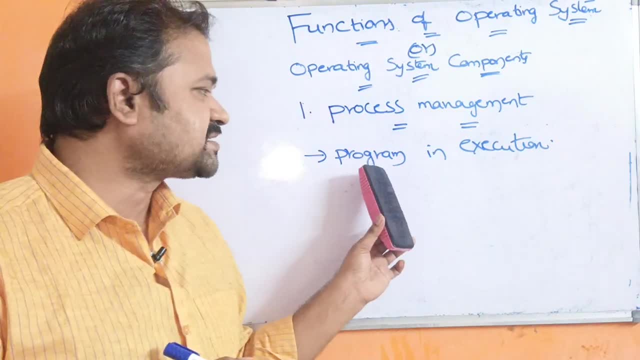 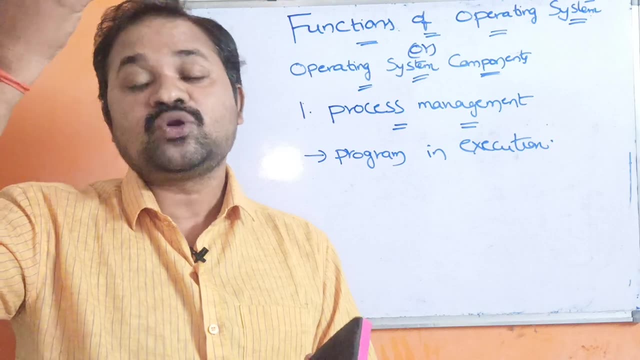 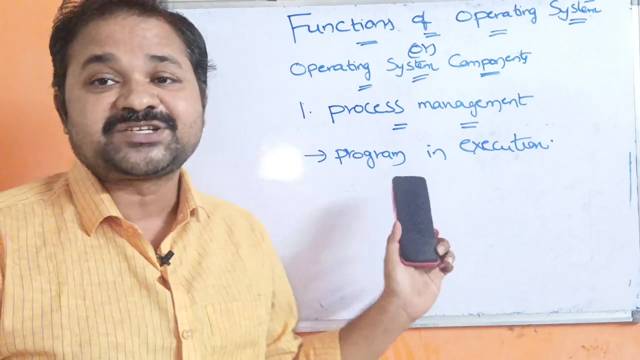 is called as process. so what is a process? process means a program in execution. so during execution, operating system loads the program from hard disk into the main memory. so if the program is loaded into the main memory, then it is called as a process. okay, so this is the definition for the. process. now let us see what are the functions of the operating system. so, in connection with, in connection with process management operating system do several activities. the first one is operating system: create a process. operating system- create a process in connection with process management operating system will do all these activities. okay, it creates a process and it also suspend. 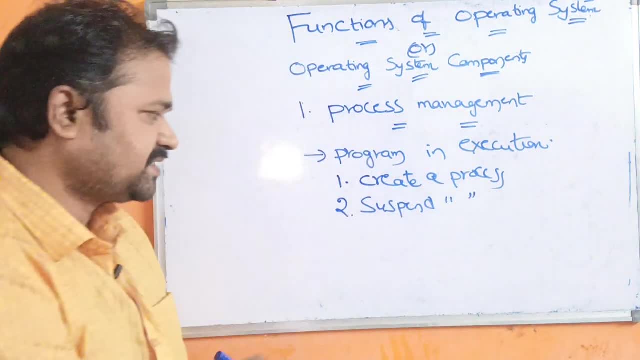 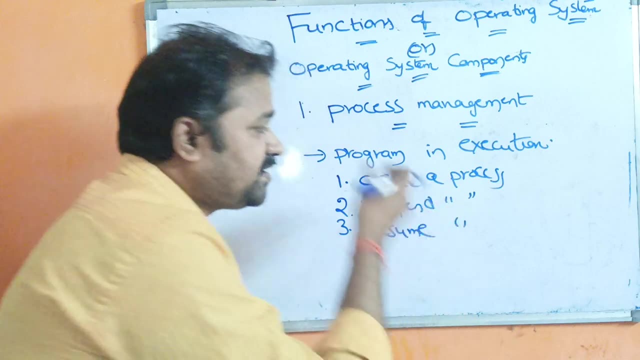 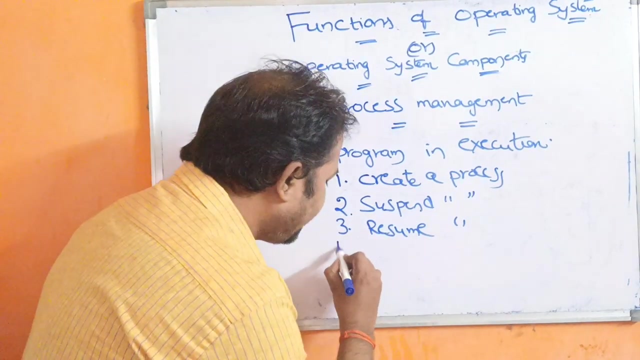 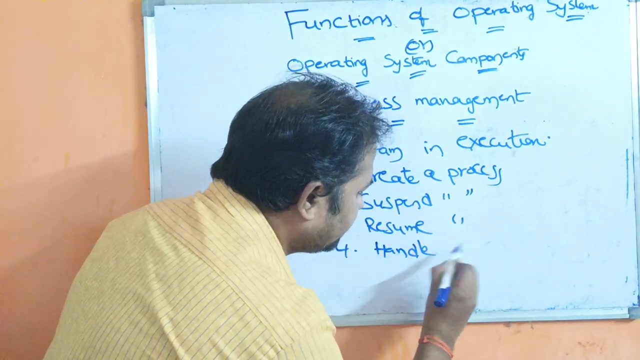 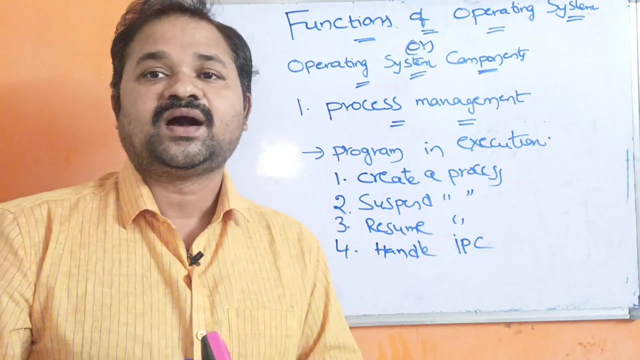 your process. if the program requires a my operation, it will suspense the process and it after suspension is over in order to resume that process. it is the duty of the operating system only to resume the process. next it will handle process communication, so handle. we have inter process communication, ipc. so ipc means inter process communication and we 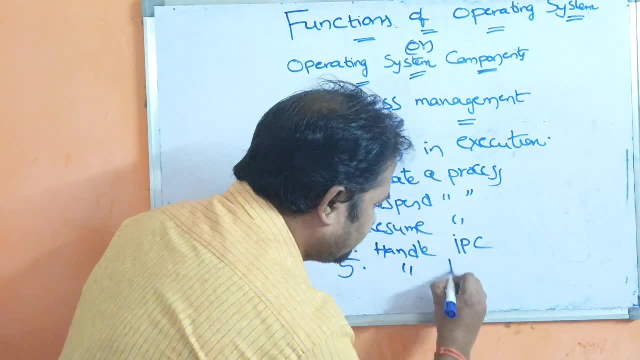 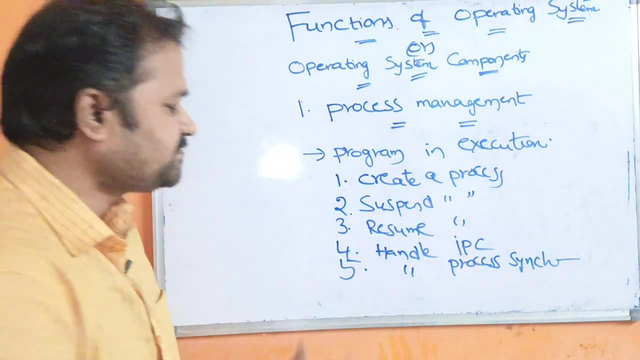 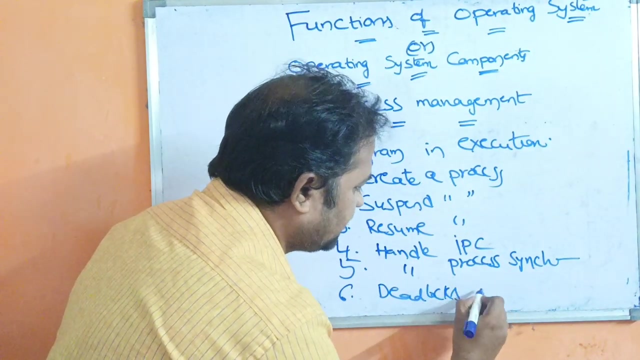 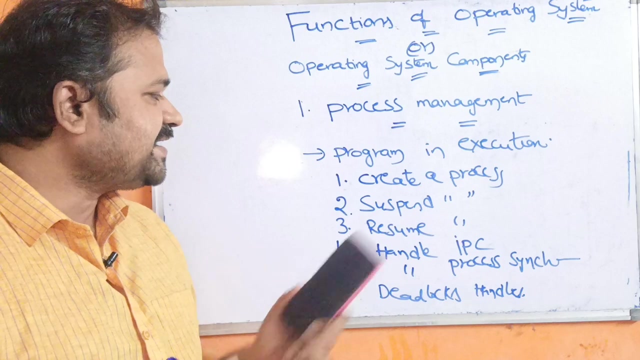 have a concept called process synchronization. so process synchronization will also be handled by the operating system only in connection with process management and deadlocks. so deadlocks also handled by operating system only. okay, so deadlocks are also handled. okay. so in connection with process management, operating system, do all these activities okay. we know that nowadays we 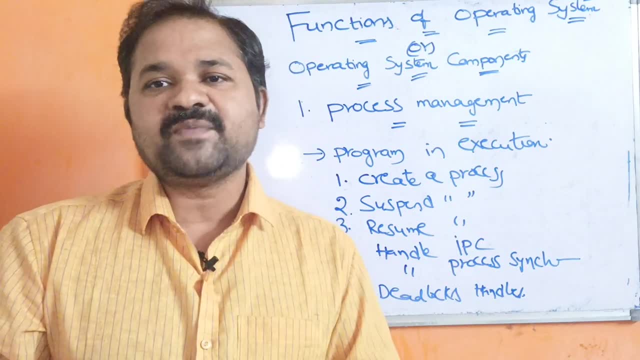 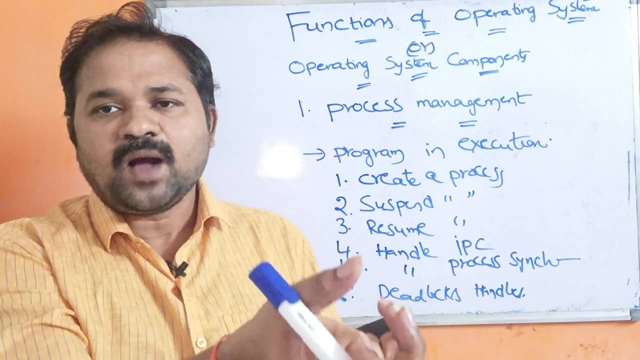 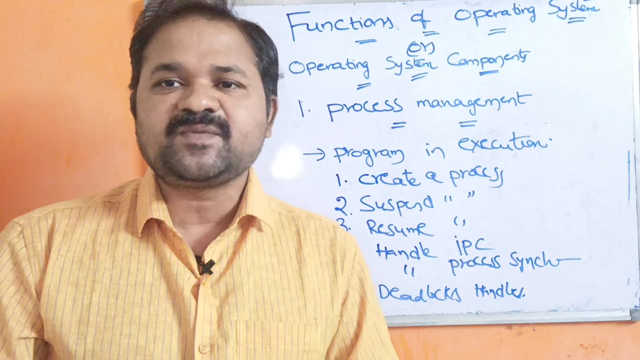 are using multi-programming system. in a multi-programming system, multiple programs- that means multiple processes- resides in the main memory. if your program is loaded into the main memory, then it is called as a process. okay, so in a multi-programming system we can have multiple processes. resides in the main memory. 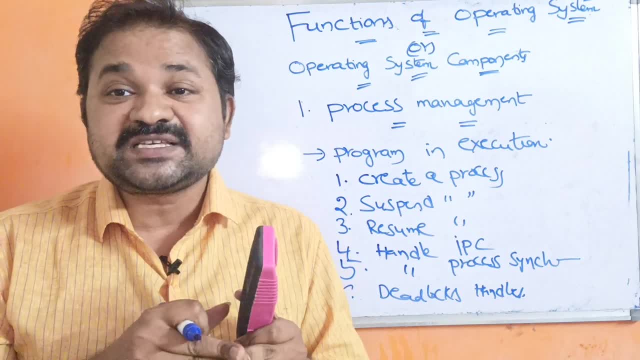 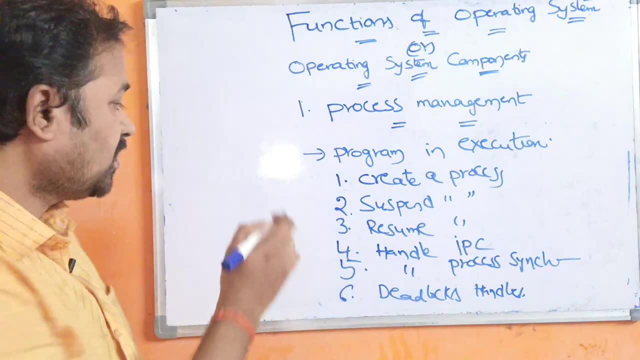 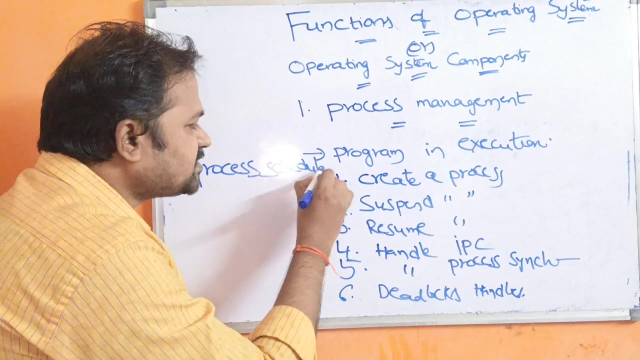 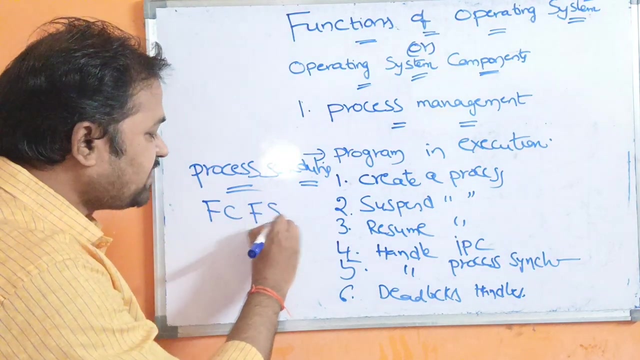 so, out of all those processes, which process we have to execute first? next, which process we needs to execute, that should be decided based upon process scheduling algorithms. so process scheduling determines in which order the corresponding processes needs to be executed. we have different types of scheduling algorithms, such as FCFS, SAF- shortest remaining time first, SRTF. 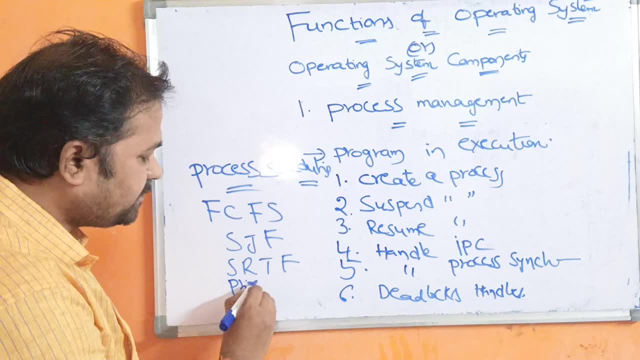 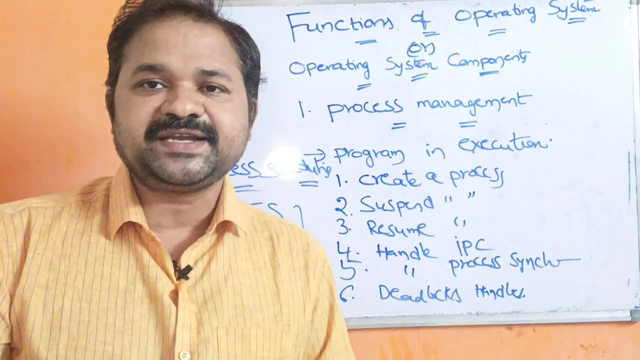 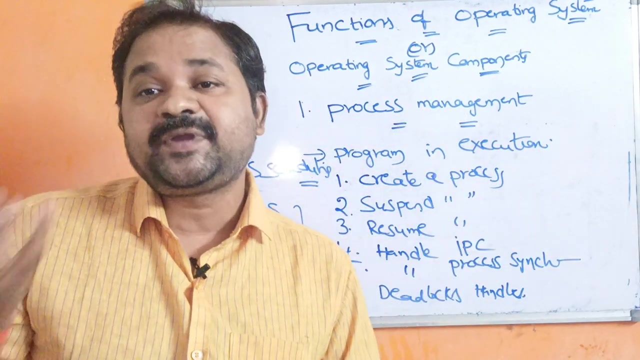 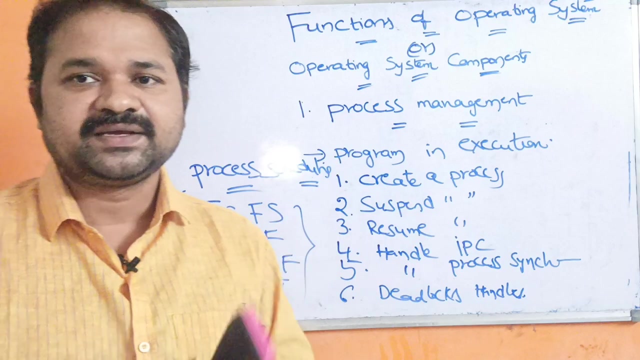 next we have priority scheduling algorithm, round robin scheduling algorithm: okay, so by using all these algorithms, operating system decides in which order it needs to execute the processes. here. process management is a chapter in operating system. subject: okay, so you can write anything available: the process: okay. in this concept: okay, it is a chapter. so we have several concepts. are there? 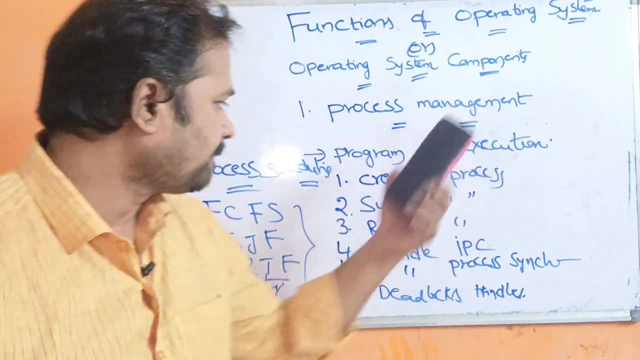 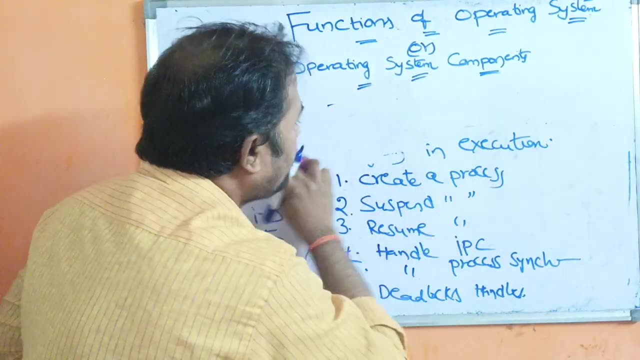 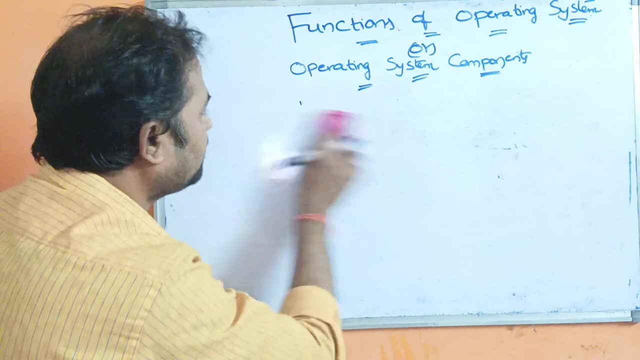 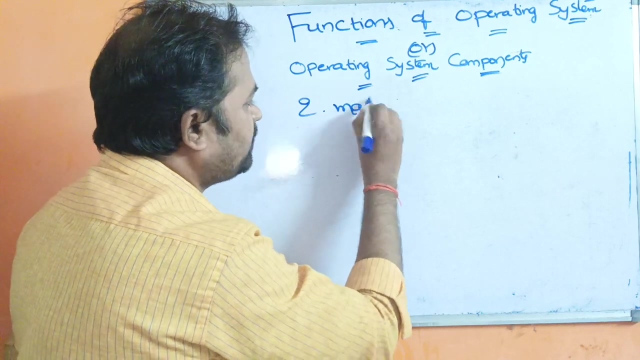 so we can explain all those concepts okay in this concept. now let us see about the second function of the operating system, or the second component of the operating system, that is, main memory management. so we have we need to handle operating system needs to handle main memory as well as secondary memory also. first let us see about main memory management. 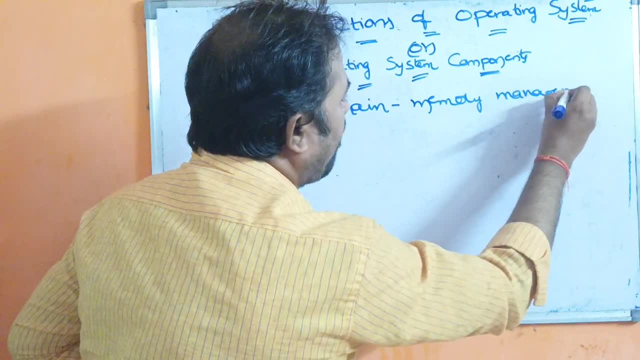 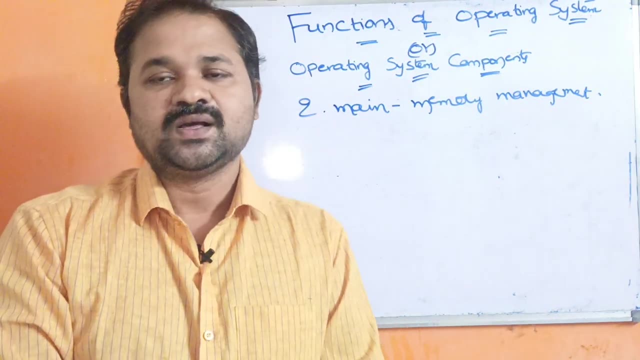 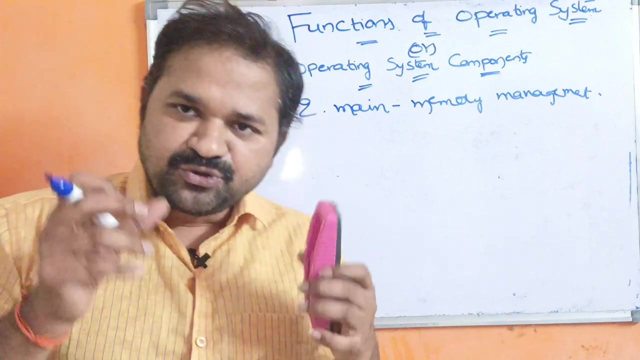 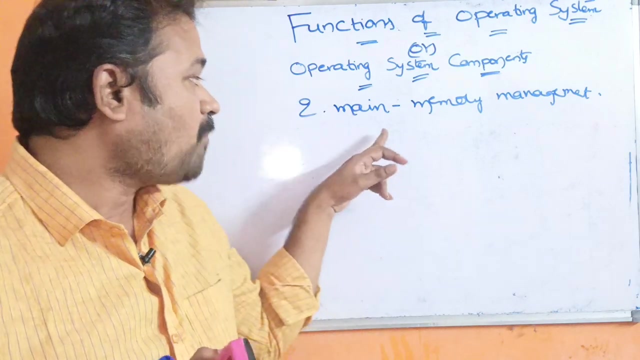 main memory management. so when operating system loads the program from hard disk into the main memory- already we have seen that point. okay, so after saving the program the program resides in hard disk only, but so during compilation also the program resides in hard disk only, but at the time of execution operating system loads the program from hard disk into the main. 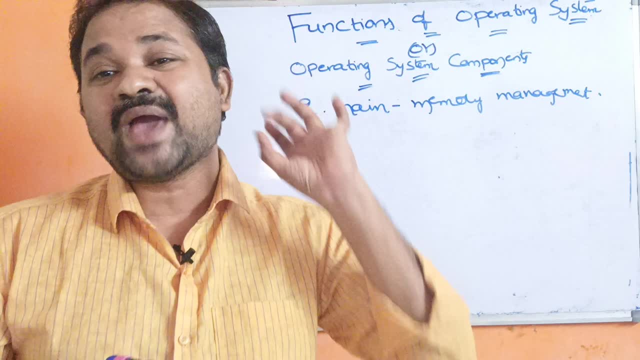 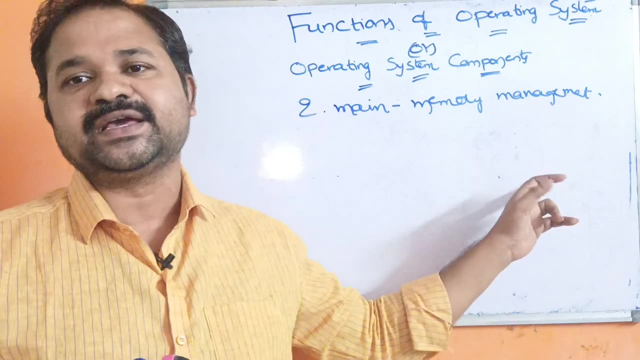 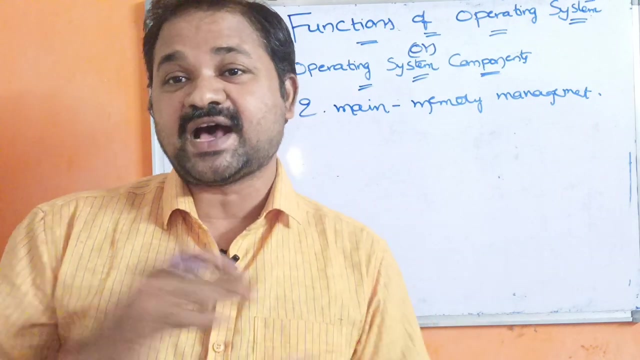 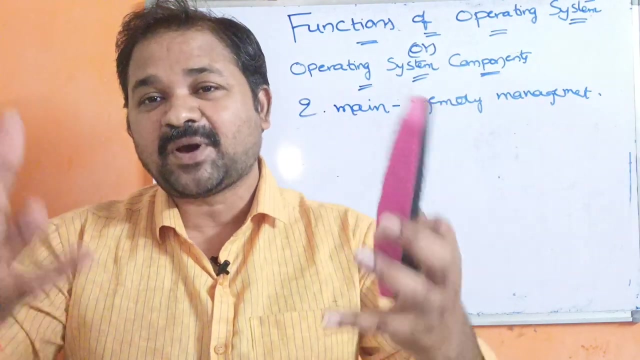 memory. why? because cpu has to execute the process or program, but cpu can access only main memory only. cpu cannot access hard disk, cpu cannot access secondary memory. so that is the first task here. okay, in connection with the main memory, management operating system mainly performs some activities. the first activity is during execution. 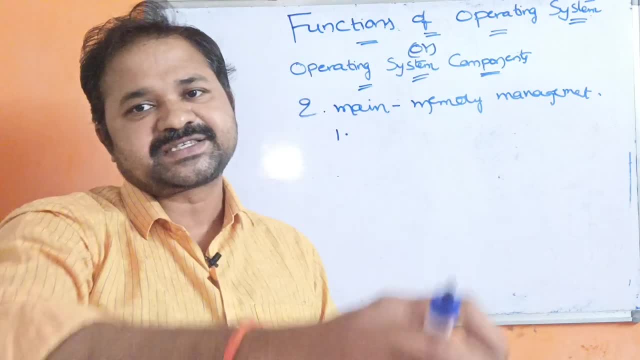 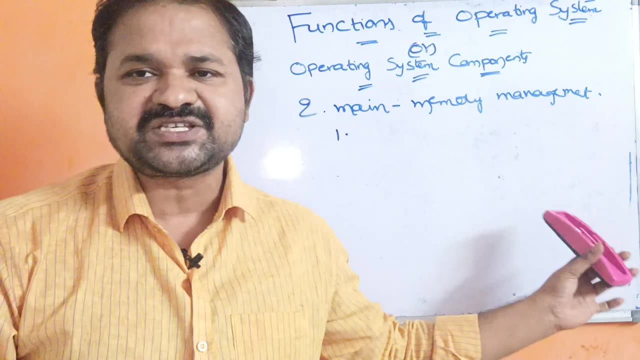 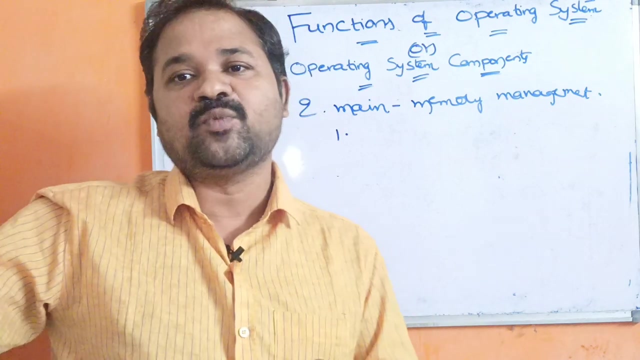 operating system loads the program from hard disk into the main memory. so for that purpose it uses several allocation techniques. we will discuss those techniques later. okay, so this is the first one. operating system loads the program into main memory from the hard disk during the execution. okay, next. 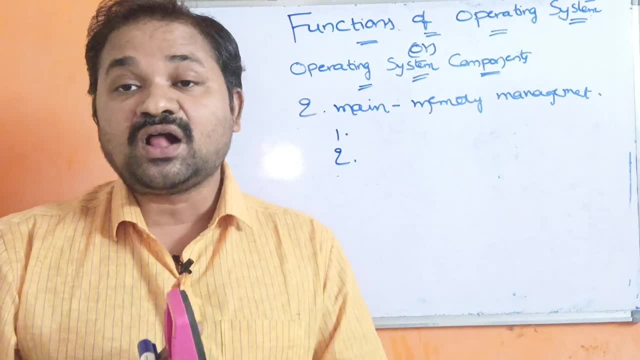 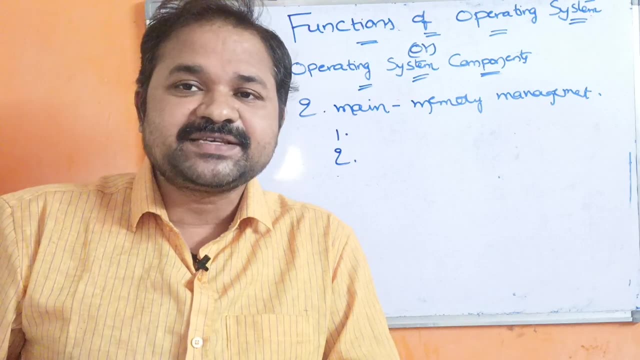 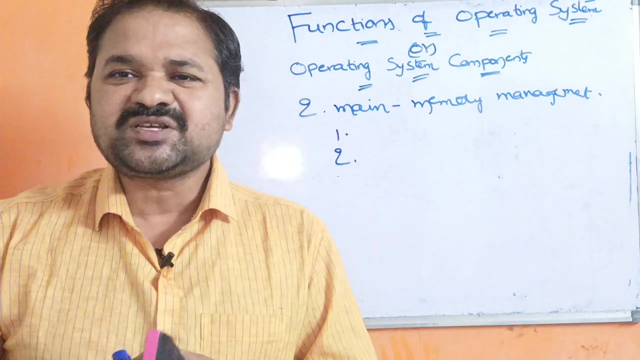 once all those operations are over. once all those operations are over, it de-allocates the memory. so that means once again the operating system has to transfer the program from main memory to the secondary memory. why? because the size of the main memory is very, very small, whereas the size of the 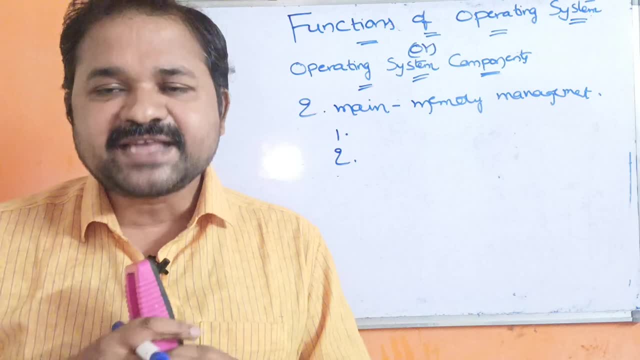 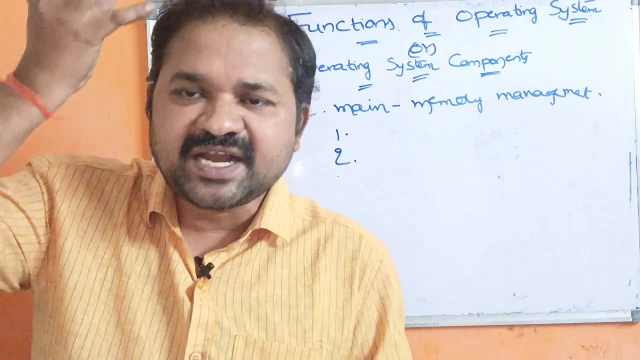 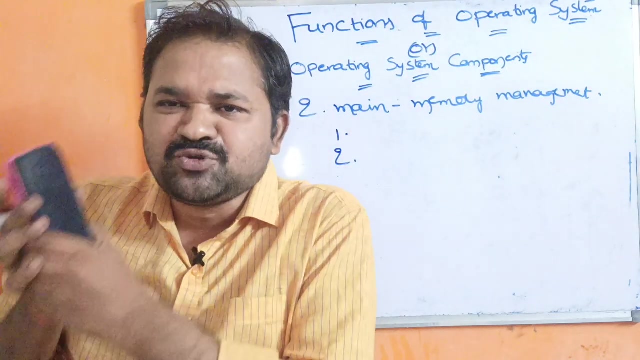 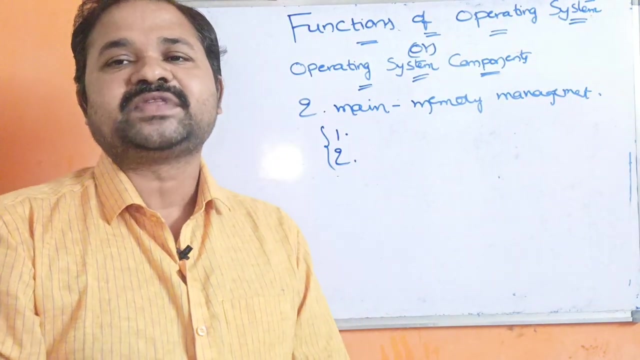 hard disk is extremely larger. so once the execution is over, once the execution is over, operating system has to has to transfer that program, that process from main memory to the secondary memory so that operating system may use that space in order to store some other programs. okay, so these two are the major activities that the operating system will do in connection with. 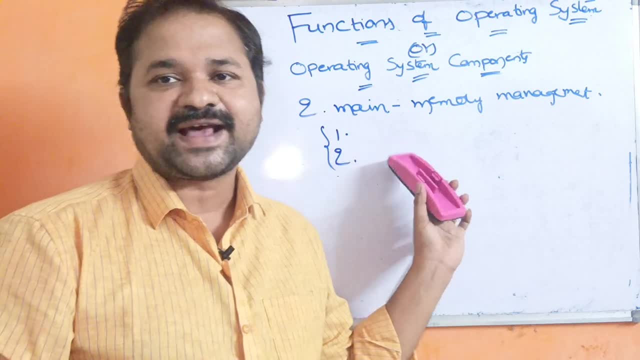 the main memory management. so the first activity is transferring the program from hard disk to the main memory and the second activity is after execution is over. it once again has to do some. save this password and then you will learn how to turn off the master token beyond the high". 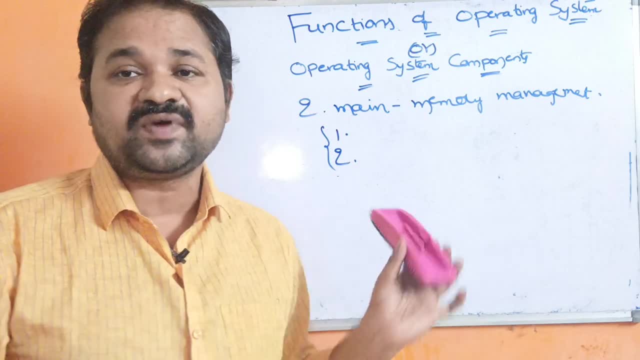 Geraki whatsapp 어느tes. that's important to learn before you start the program and after executing on the prettiest operating system. the second activity is after execution is over. you will learn after today. you will learn after we kept using the second activity cái. 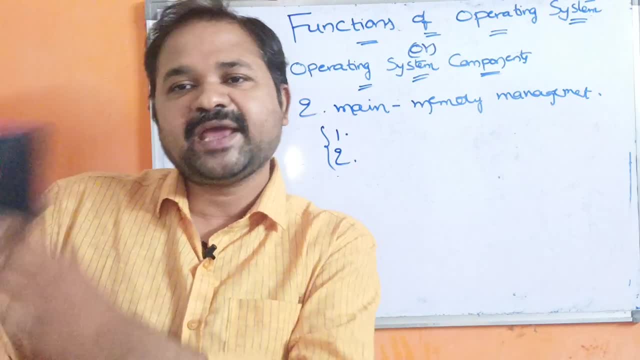 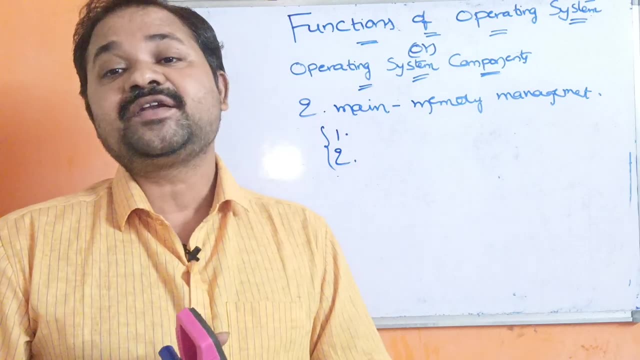 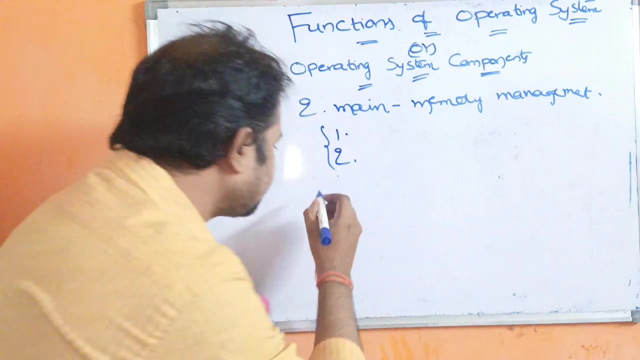 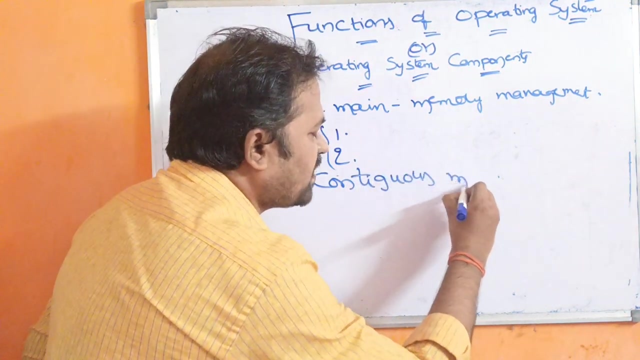 does that 음 again needs to transfer that process from main memory to the secondary memory. now let us see how the operating system will allocate the memory. in order to allocate memory for the corresponding process, operating system mainly uses two approaches. the first approach is contiguous memory allocation. the first approach is contiguous memory allocation in contiguous memory allocation. 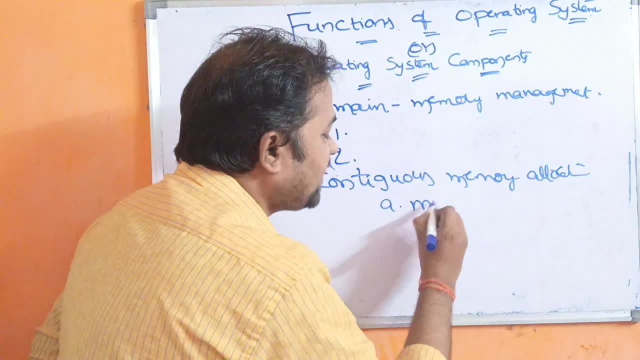 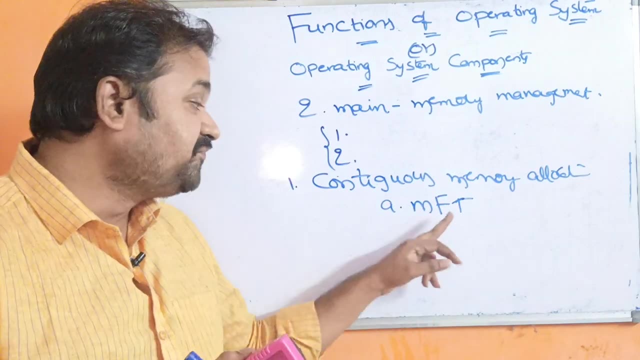 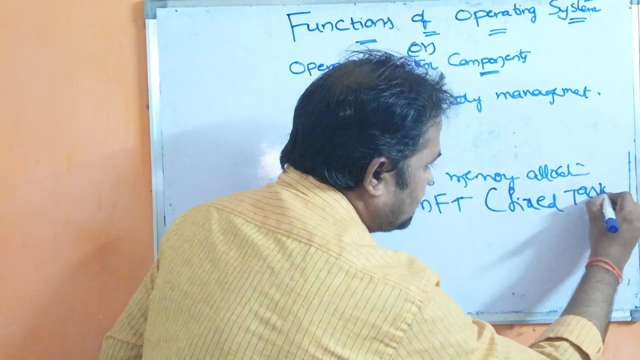 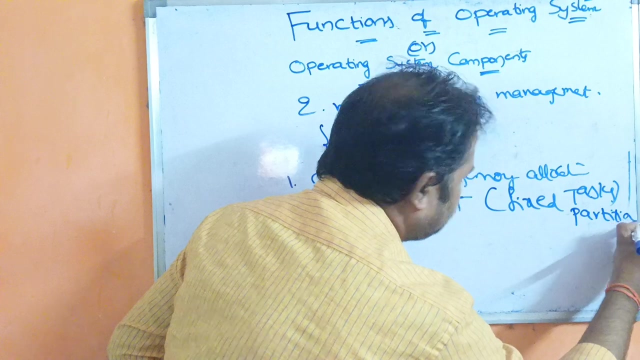 we have two approaches are there. first one is mft. mft stands for multi-programming, m stands for multi-programming with f stands for fixed fixed, t stands for tasks. so multi-programming with fixed tasks, or we can also call it as fixed partitions. and the second approach is mvt. 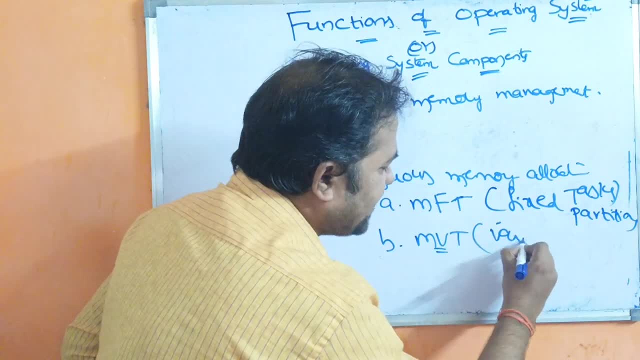 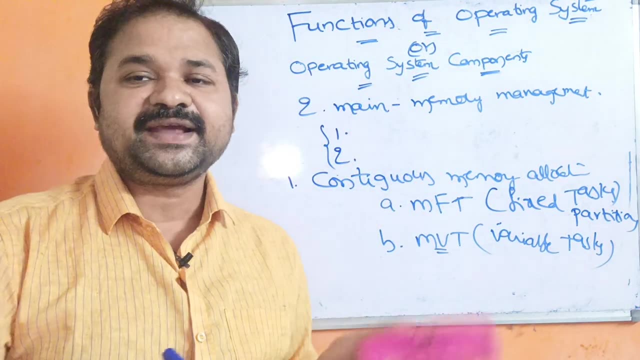 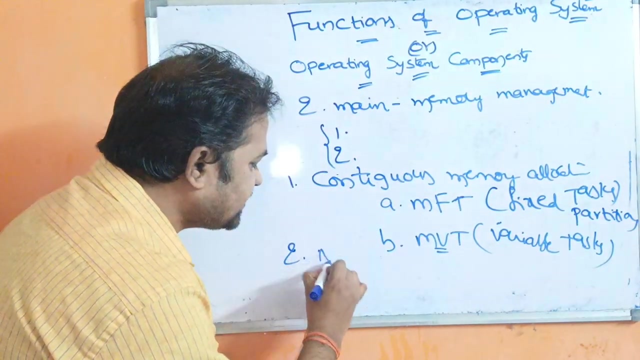 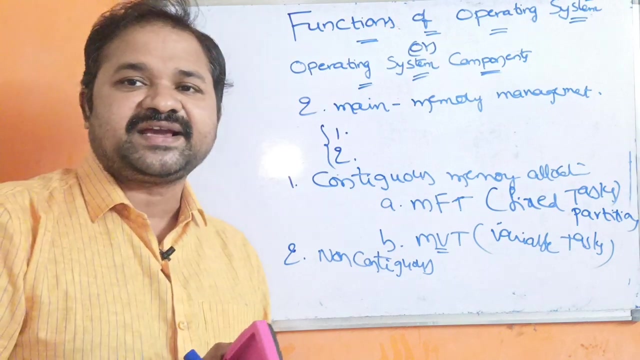 multi-programming with v stands for variable, t stands for tasks. so in the olden days operating system uses these two, this approach, whereas nowadays operating system is using the second approach. that is nothing but non-contiguous allocation. non-contiguous allocation for non-contiguous allocation. 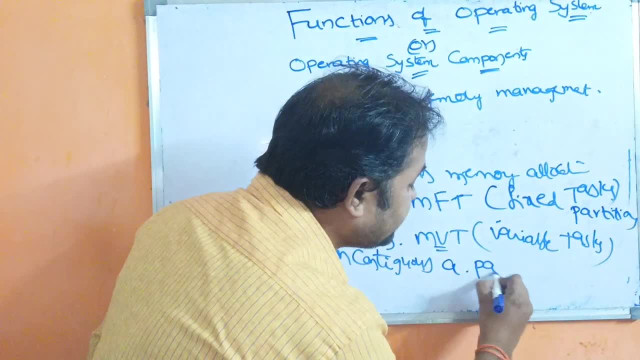 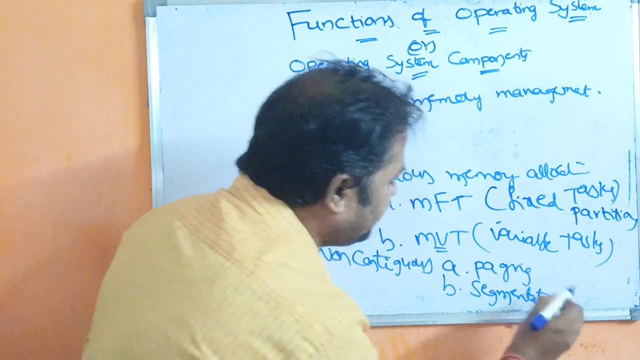 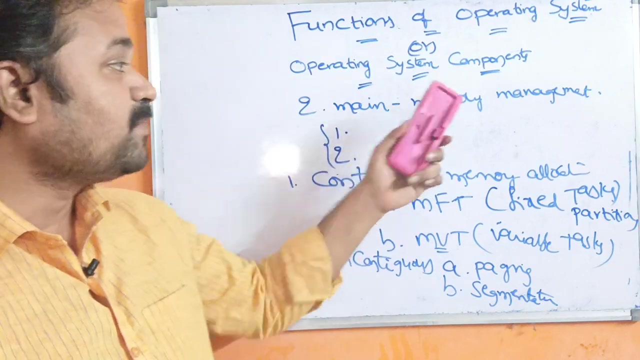 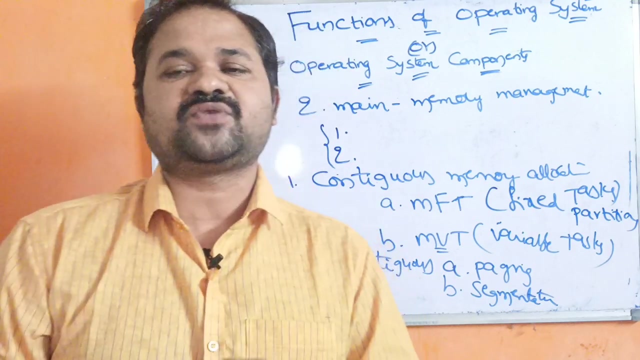 the best examples are: the first example is pacing- pacing. the second example is segmentation. the first one is pacing, second one is segmentation. so these two are the non-contiguous memory allocation techniques. okay, here, main memory management is a chapter in operating system. so once you understand all those concepts of the main memory, then you can write more, more points. 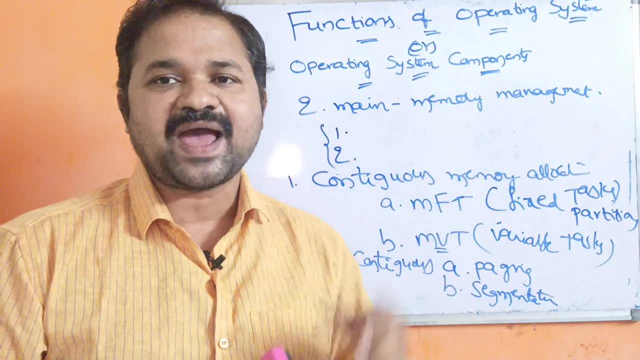 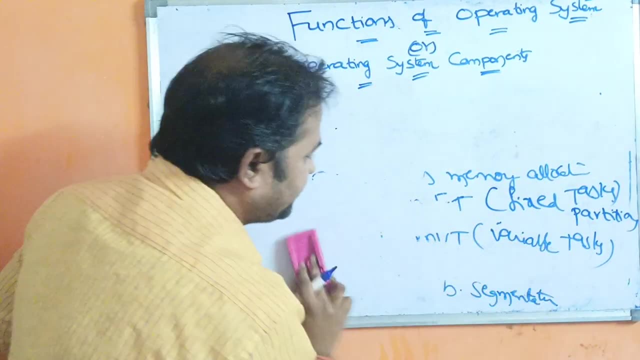 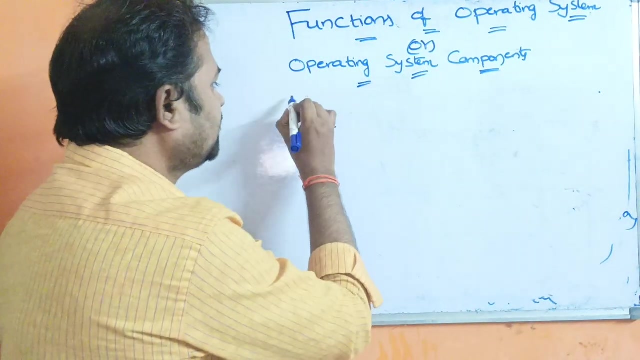 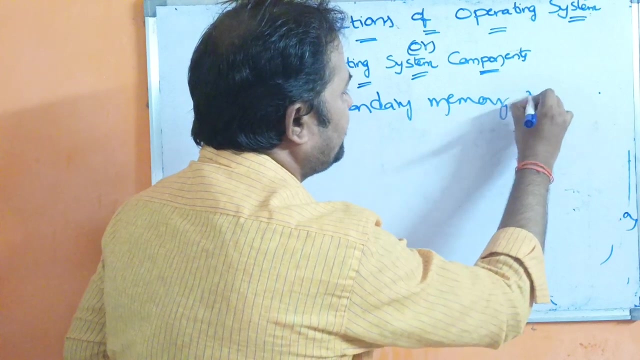 here also: okay. so in this way operating system handle main memory management. now let us see the third one, that is, the main memory management. so in this way operating system handle main memory management, secondary memory management, secondary memory management. how operating system handles the secondary memory. okay, so this is monotopic, only secondary memory management, secondary memory. 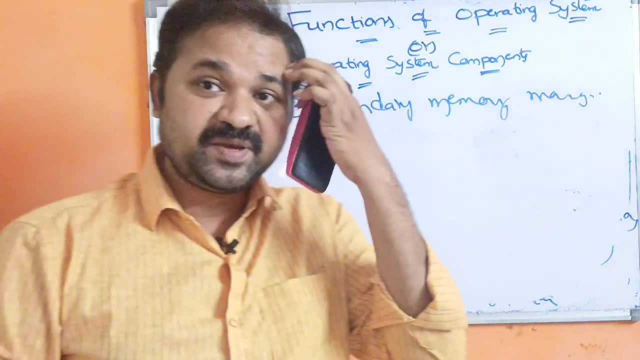 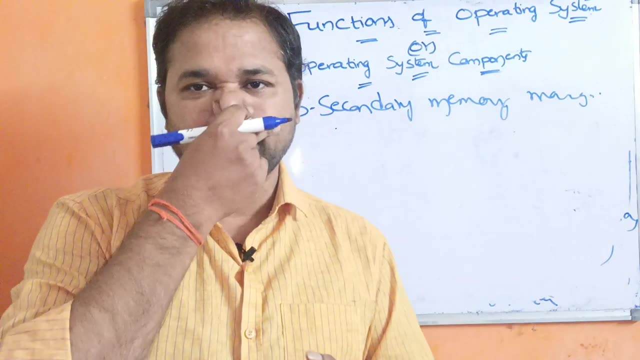 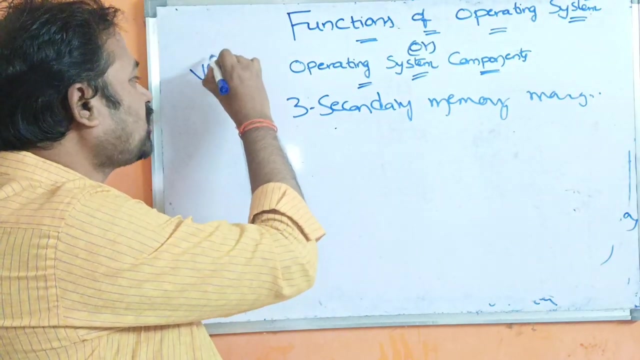 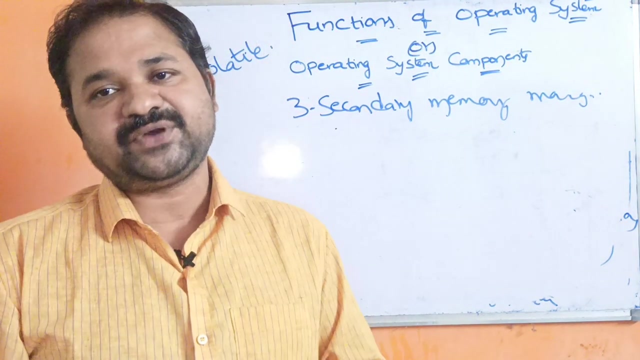 management. okay, secondary memory management. so here also we know what is the advantage of the secondary memory. already we have seen main memory. main memory means ram. main memory is a volatile memory. main memory is a volatile memory. volatile means the contents of the main memory will be lost when you switch off the computer. so when we when the power is turned off, then what will? 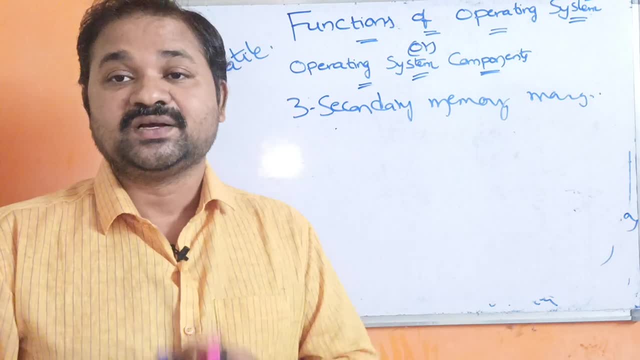 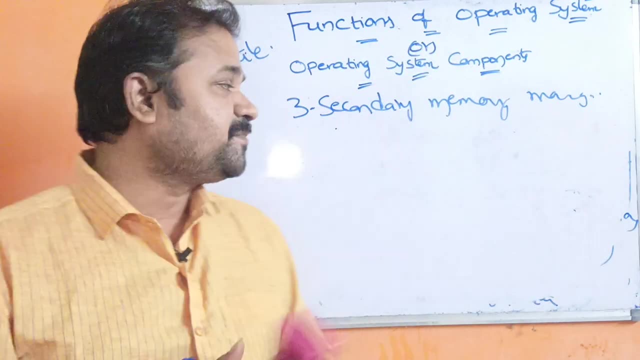 happen, the contents of the main memory will be last, so we need to have a device which stores our information permanently. so for that purpose, we are using secondary memory. the best example for the secondary memory is how to use secondary memory, how to use secondary memory. how to use secondary memory. 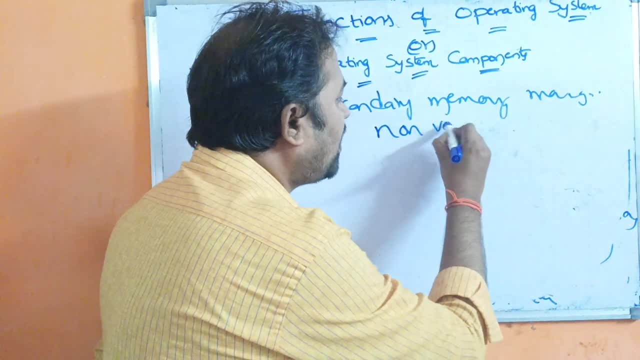 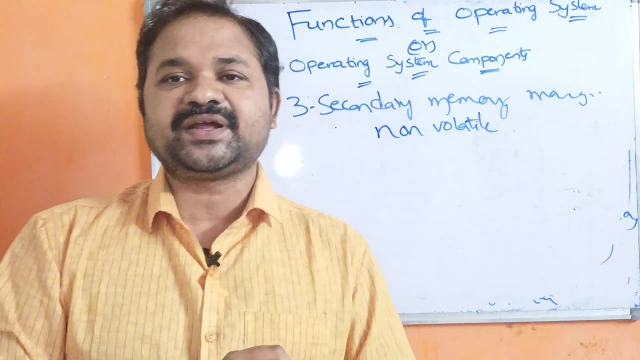 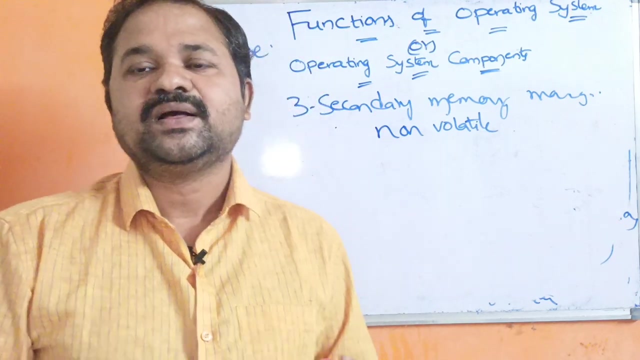 hard disk. hard disk is non-volatile memory. non-volatile means our data will be stored permanently in the computer. even though we switch off the computer, there is no problem. our data will be stored permanently in the computer. so whenever we save any program, then it is stored. 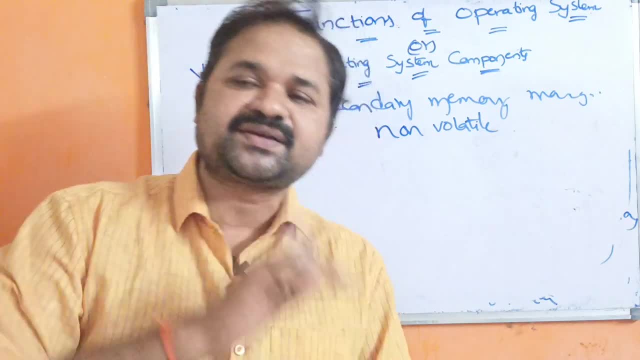 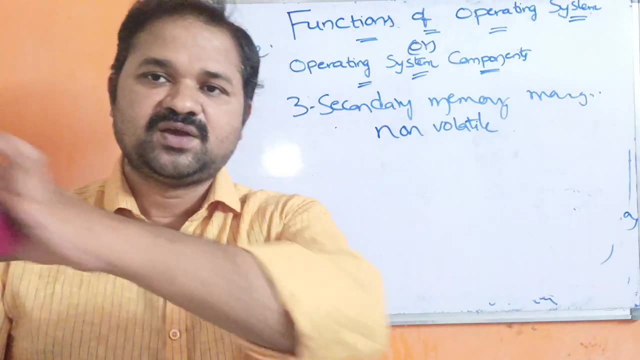 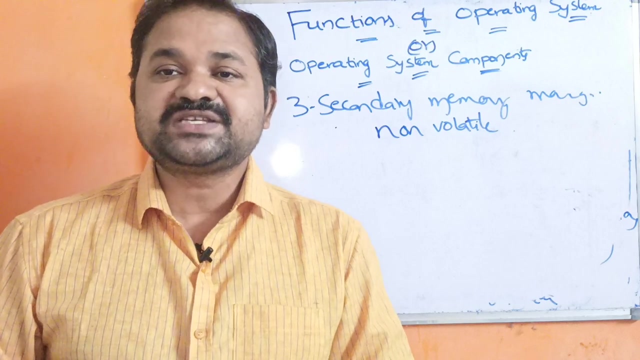 in the hard disk. during compilation also, it is in the hard disk, but at the time of execution, operating system transfers the program from hard disk into the main memory. why? because cpu can execute the program only when it resides in main memory, only after the execution is over. once again, 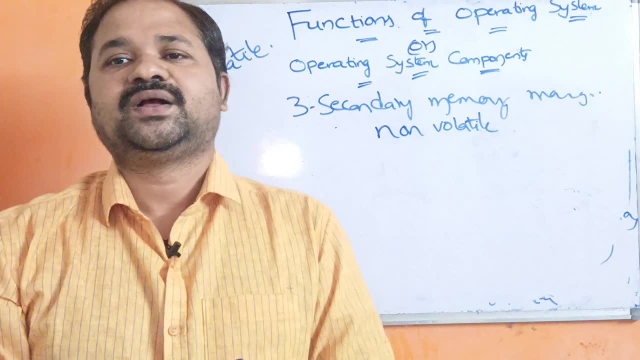 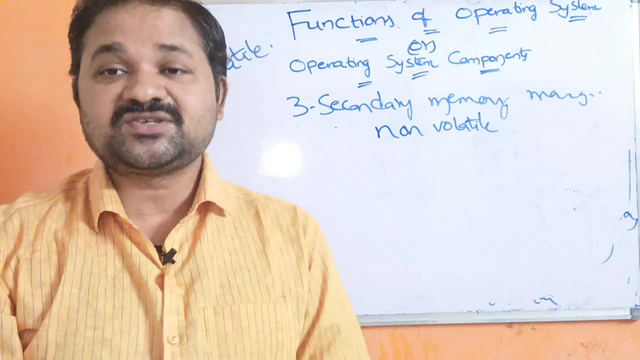 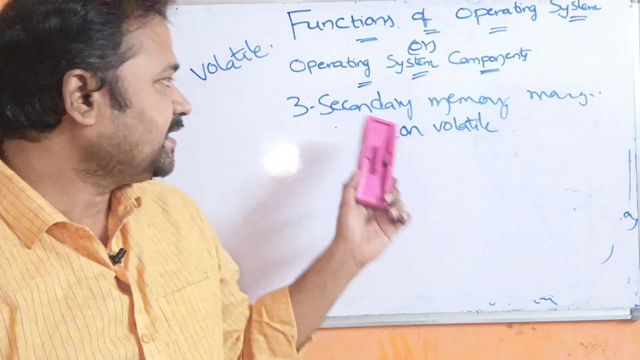 that program will be transferred from hard disk to the. i'm sorry once again. that program will be transferred from the main memory to the hard disk. okay, why? because the size of the main memory is very, very small when compared with the size of the secondary memory. okay, here, in order to 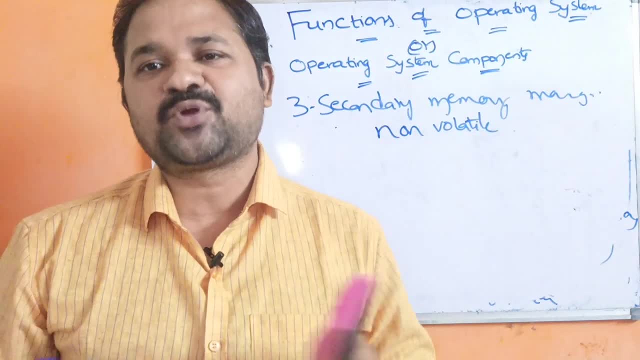 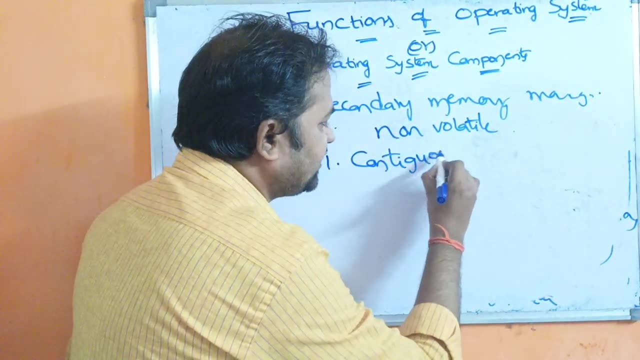 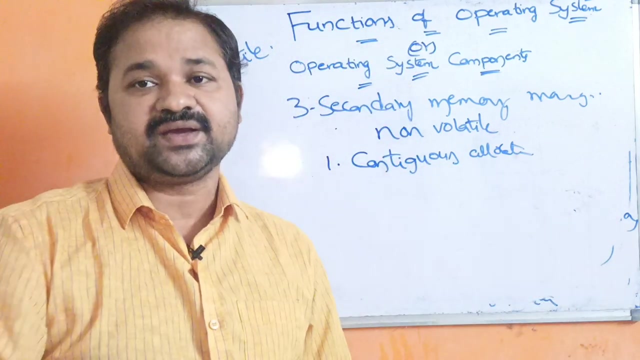 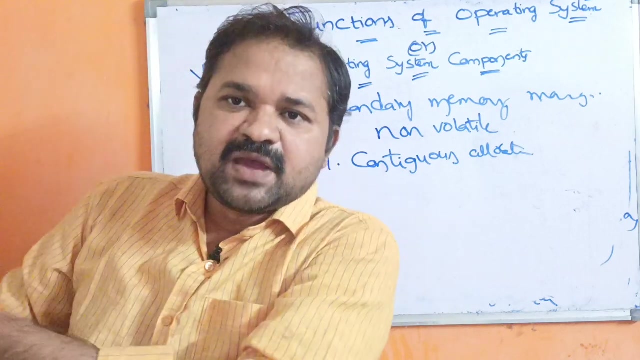 manage the secondary memory. here also we have three approaches, are there? the first approach is we have contiguous allocation. contiguous allocation: so by using this approach operating system can stores the corresponding program in the hard disk. okay, so when it will saves after the execution, that program will be transferred from the main memory to. 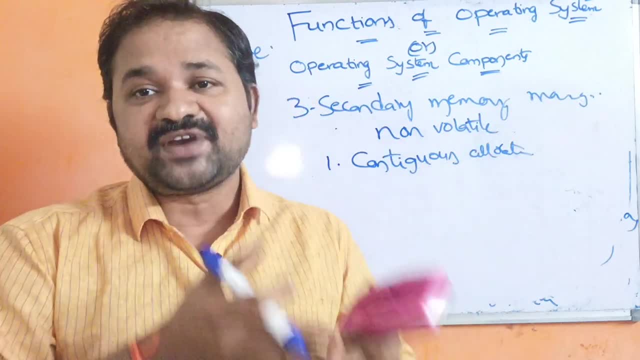 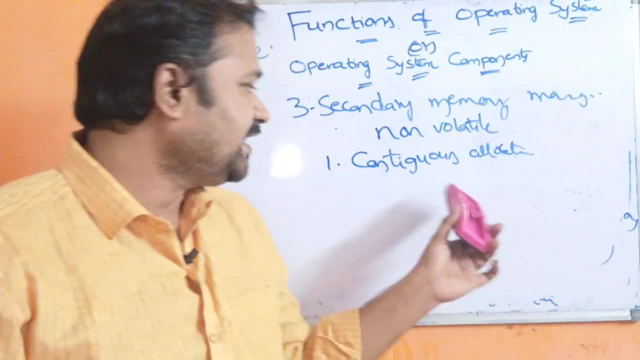 the hard disk, or initially, initially, after typing is over, we have to save the program. so in those two occasions for saving the program, we have to save the program. so in those two occasions for saving the program into the hard disk, it uses contiguous allocation. next one is link list allocation. 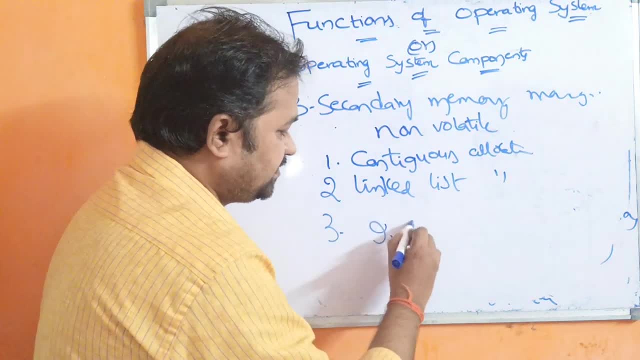 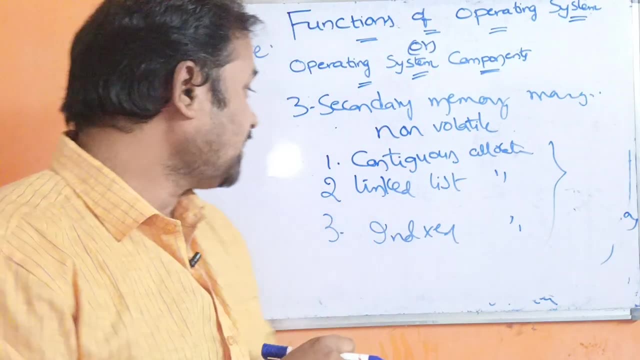 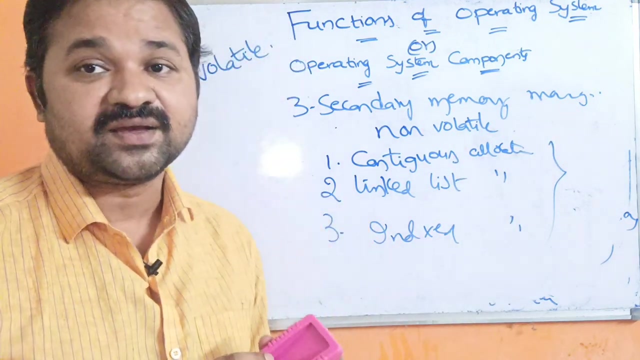 link list allocation. third approach is index delegation. index delegation: mainly, it uses these three approaches in order to store the data in the, in order to store the data in the corresponding secondary memory. so in this way operating system handles secondary memory. we have a chapter called disk management. okay, there you will get. 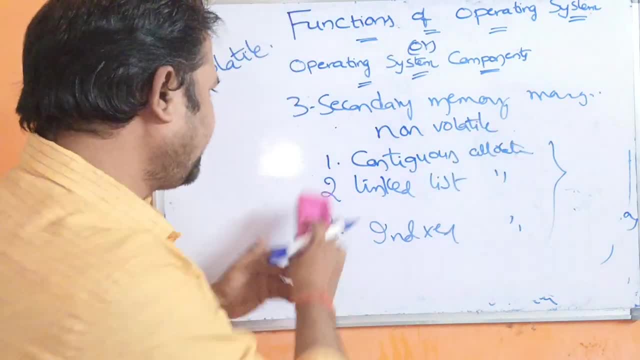 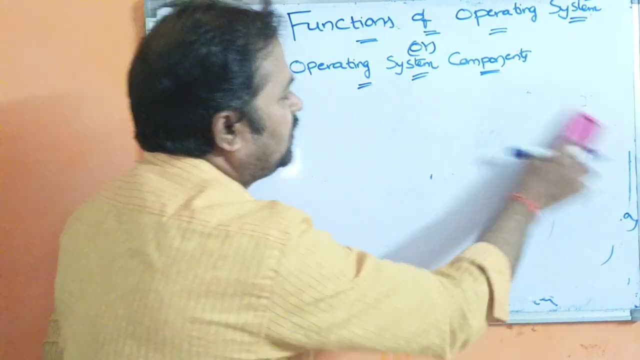 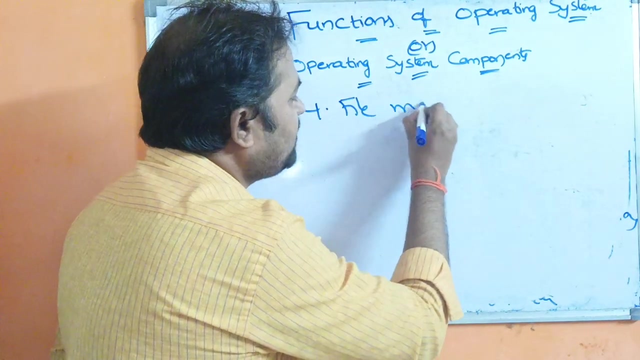 some more idea about secondary memory management. okay, so this is also a chapter in the operating system. so once you understand that, those concepts, then you can write more points. okay, and the fourth function of the operating system is file management. file management- let us see what is a. 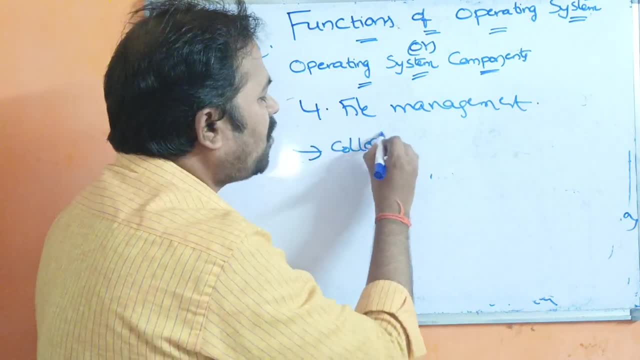 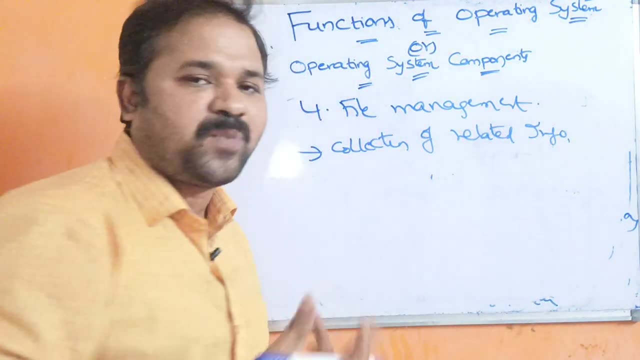 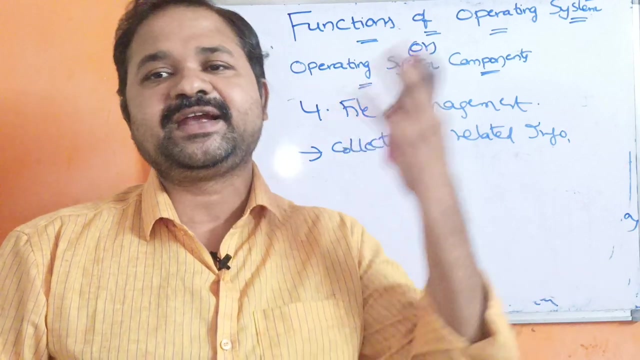 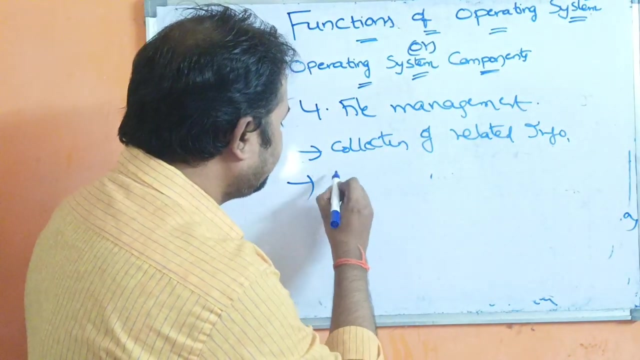 file. so file means a collection of related information. so file means a collection of related information. if you take employee file, employee file contains employee related information. if you take student file, it contains student related information. and we have some more points regarding files. also there, a file means a collection of. a file contains a collection of. we can have words. 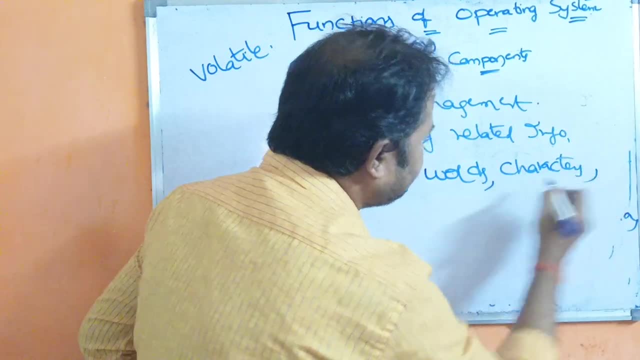 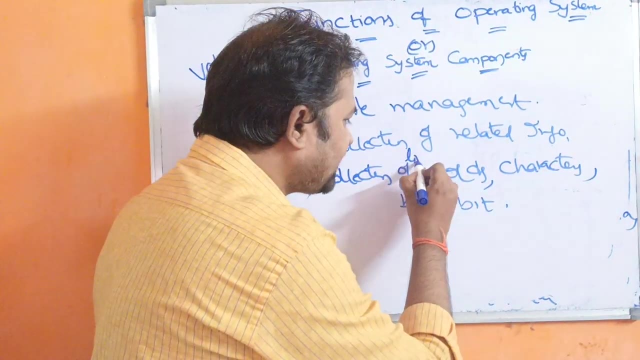 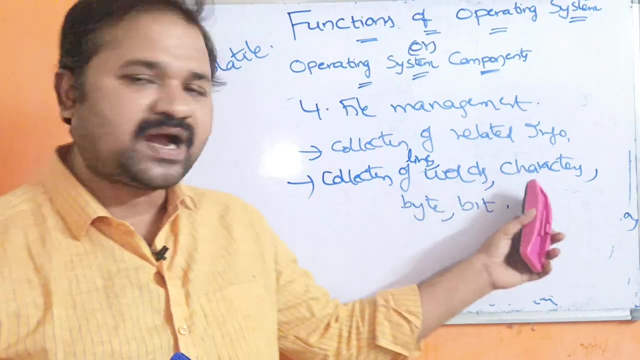 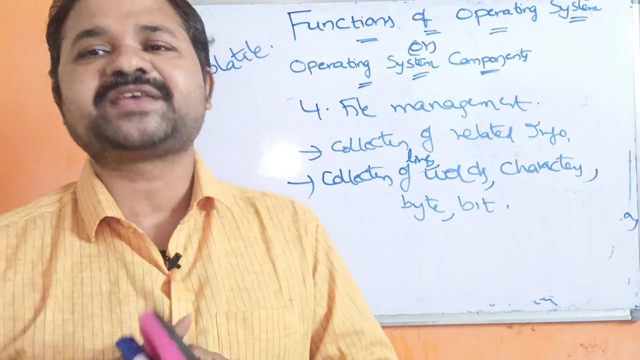 and characters: bytes, bits, bytes, bit. so a file is a collection of words or, before this, we can write line. a file is a collection of lines, where each line contains a collection of words. every word contains a collection of characters. each character is a collection of bytes. byte is a collection of bits, okay. so file means a collection. 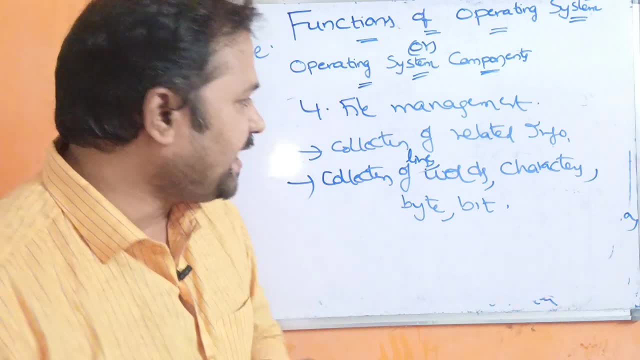 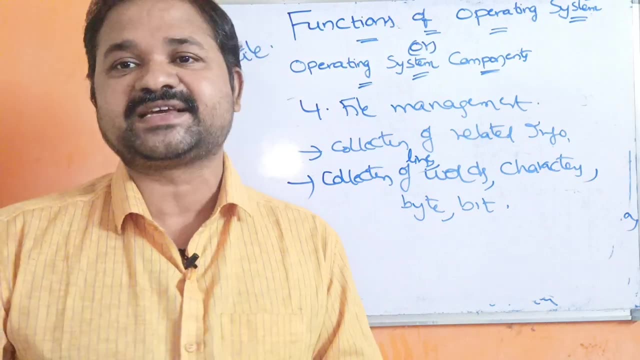 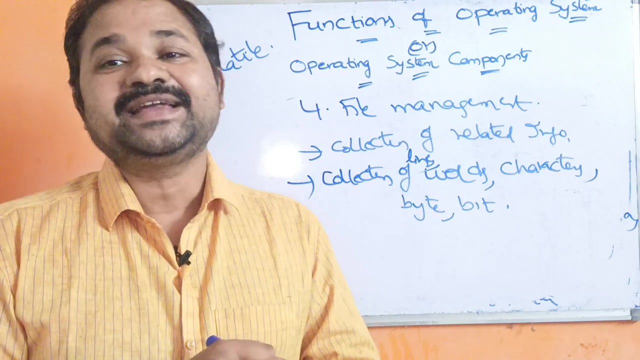 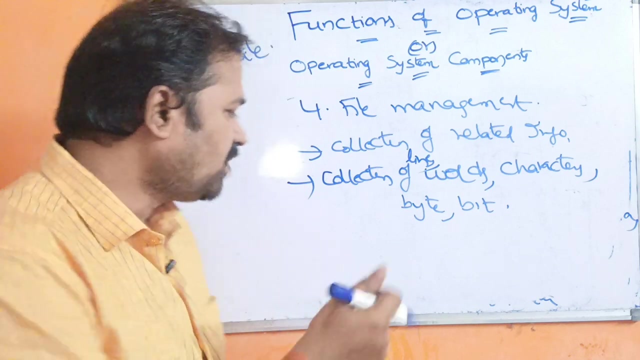 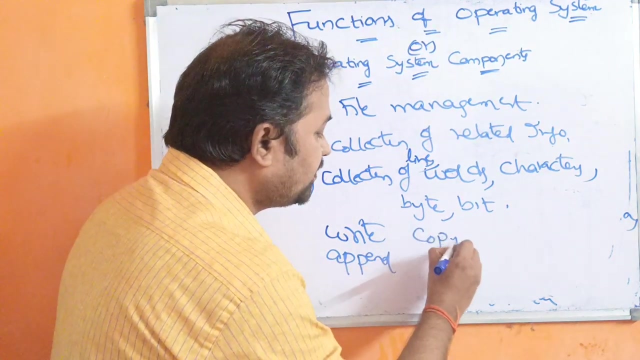 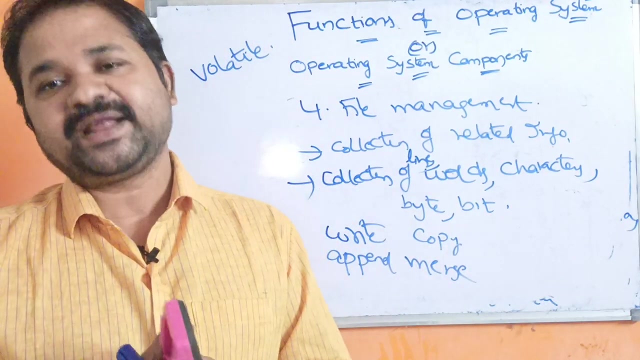 of lines, words, characters, bytes and bits. okay, in connection with file management, operating system do several activities such as creating a file, deleting a file, creating a directory, deleting a directory, opening a file, open operation, read operation, read operation, write operation. next, append operation, copy operation, merge operation, merge operation. likewise, operating system perform various operations on the files and the directories. 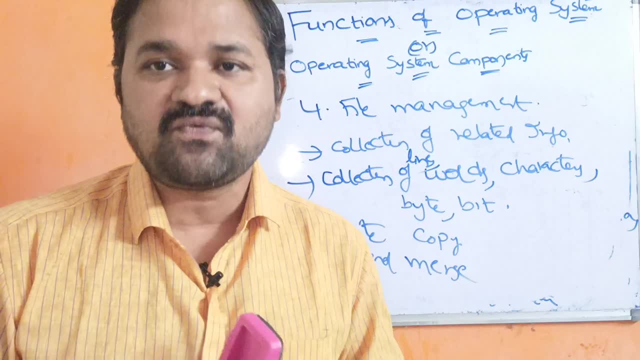 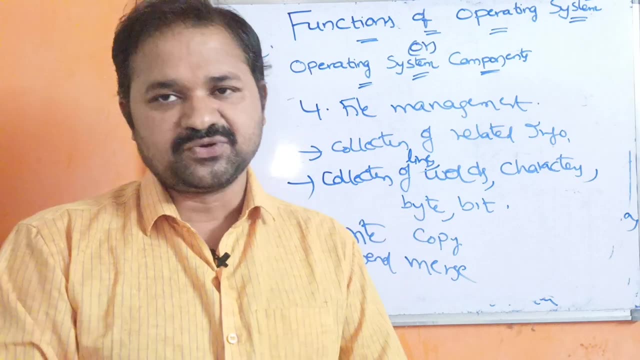 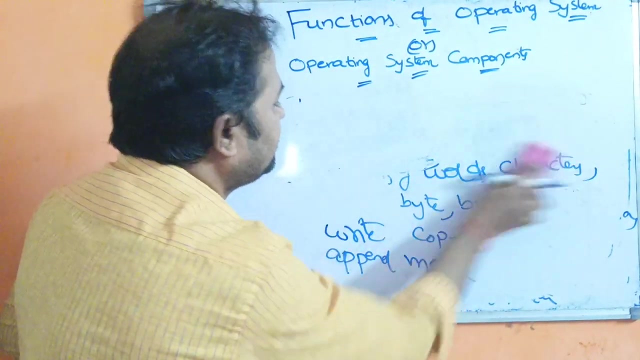 okay, we know what is a directory. directory means a collection of files. if you want to organize hundreds of files, thousands of files, then directories are used. okay, so in this way operating system handles file management. now let us see the last one, that is, io management. io management or io. 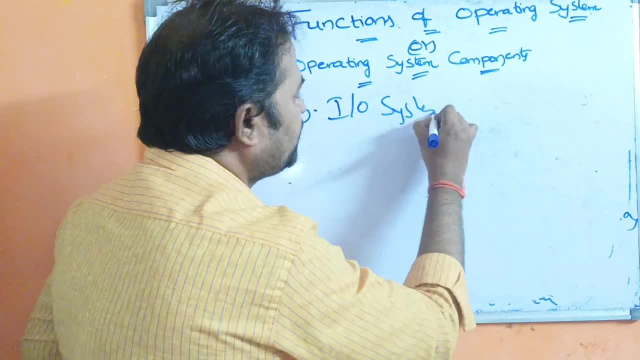 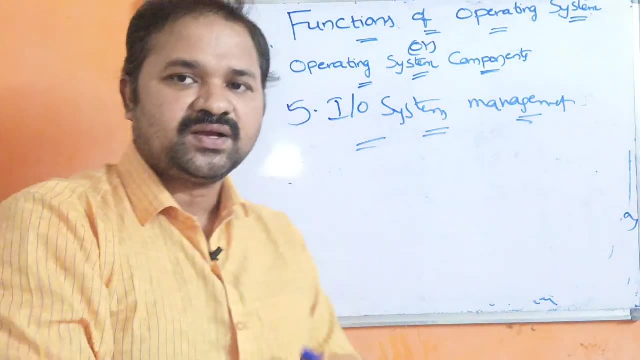 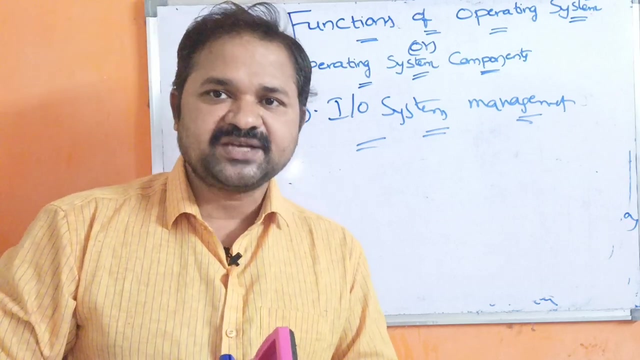 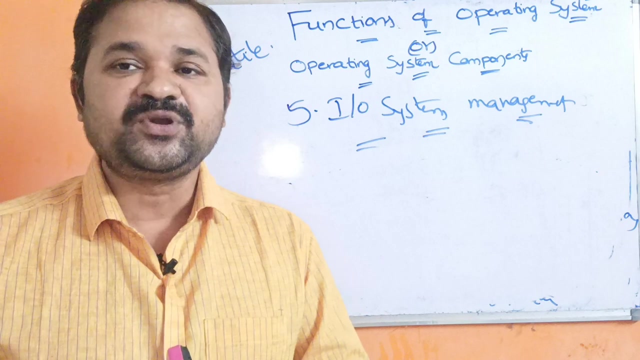 system management, io system management. so we know what is io. io stands for input and output devices. so input devices are useful in order to provide information to the computer. various output devices are useful in order to display information on the computer. for displaying we use output images, whereas for inputting purpose we use input devices. so the commonly used input 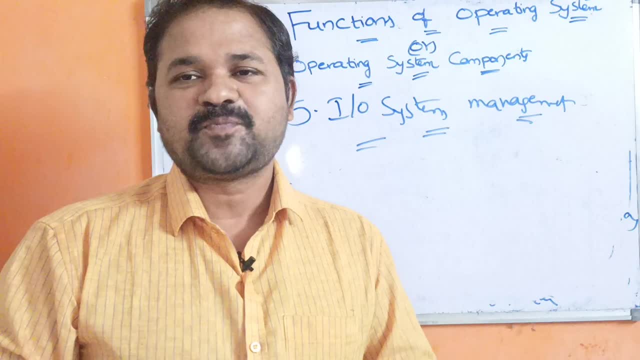 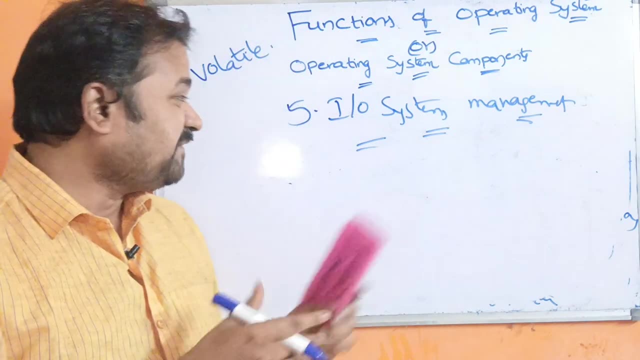 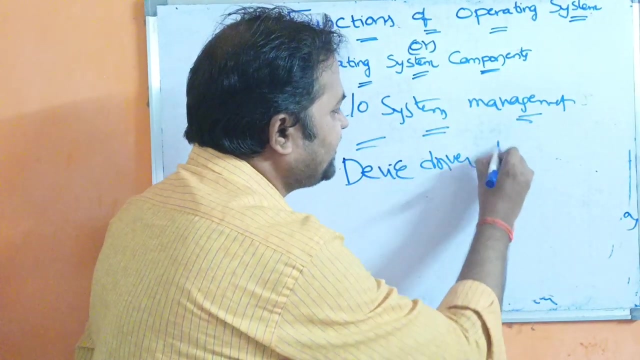 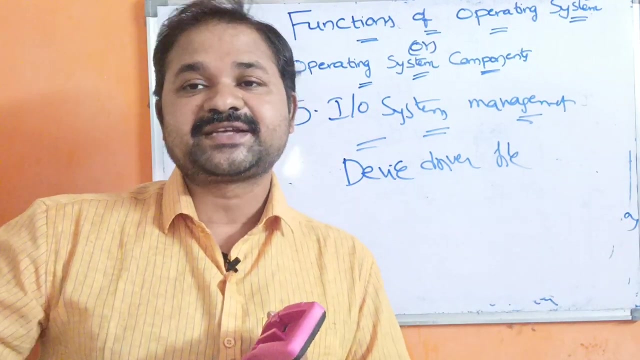 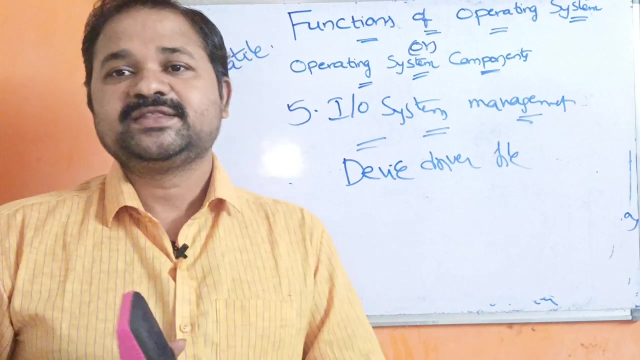 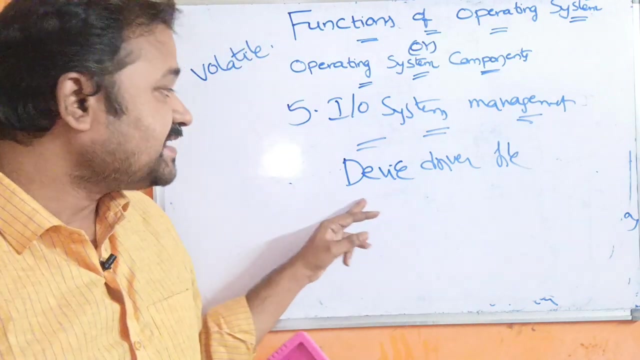 devices are keyboard, mouse, scanner, pointer. these are the commonly used input devices. the commonly used output devices are printer and scanner. okay, here, every input output device is a printer and a scanner. every input output device contains a device driver file, a device drive value vitaling for the Pi system right in 시간이 out. then it is the responsibility of the operating system to allocate the printer. so for that purpose, first, operating system sends a signal to the device driver: printerila: yeah, we are going to print it out. so for the purpose, first, operating system sends a signal to the device driver: printer is the printer. that adoption depends on it.